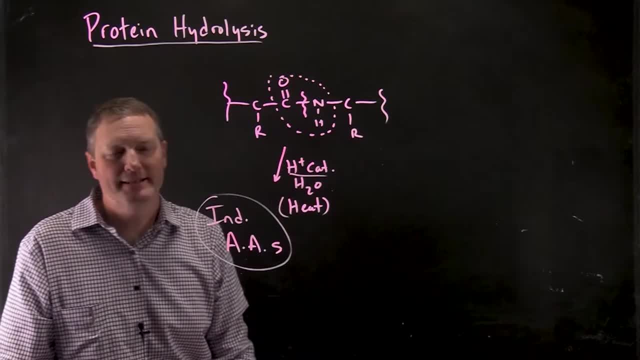 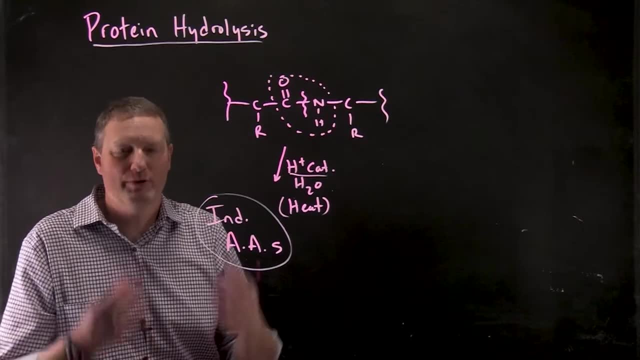 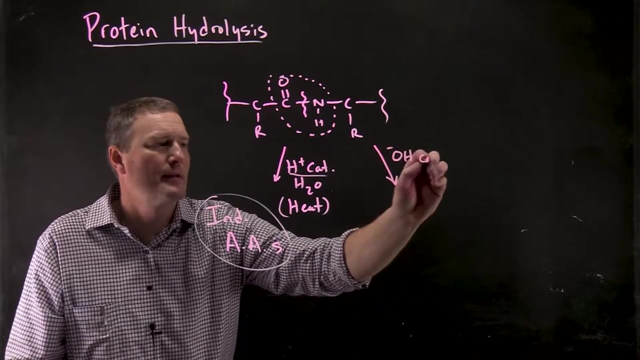 primary structure. if you were to hydrolyze that using acid-catalyzed hydrolysis, you would then get 300 individual amino acids, So you can certainly do that with strong acid and heat. You can also do this using base-catalyzed hydrolysis, so strong base H2O and also. 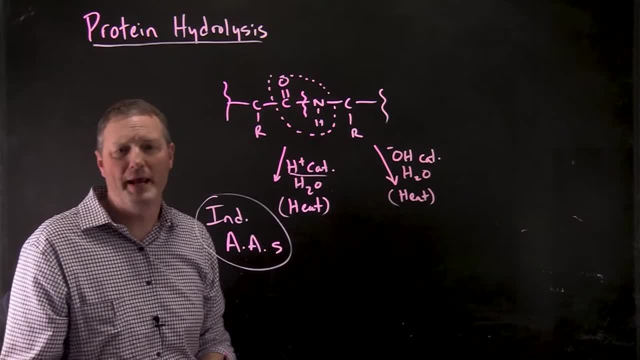 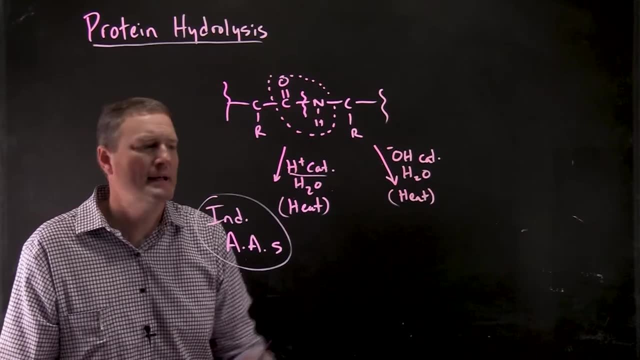 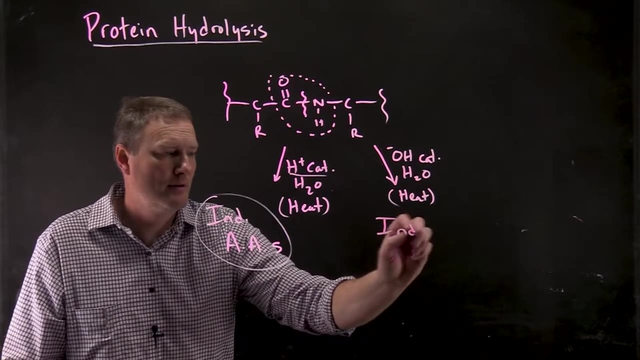 heating this, And so when I say strong base, I'm talking about like 6 to 10 molar sodium hydroxide or potassium hydroxide, and then heating this overnight Again. it would chop that 300 amino acid peptide down into 300 individual amino acids. 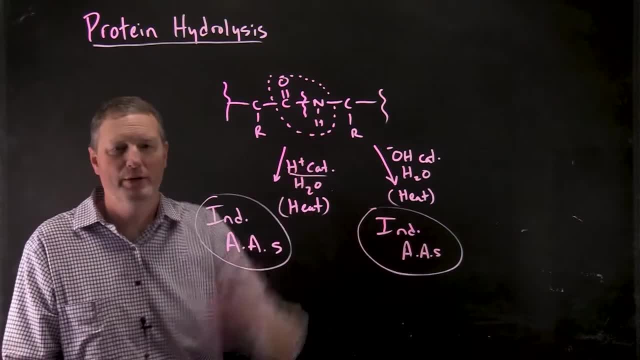 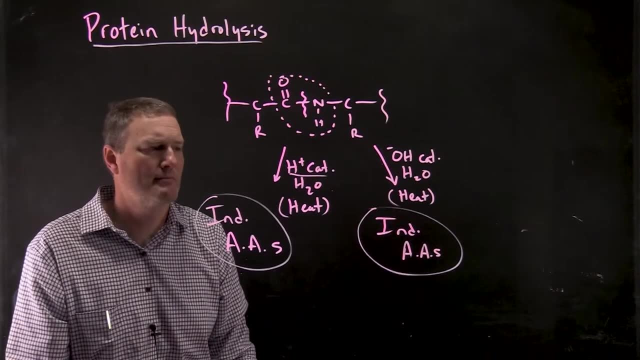 So that's how you might do this in a laboratory. If you had a protein, you could treat it with either acid or base, and then, you know, get your base. It's a sort of collection of the amino acids that are in that protein. 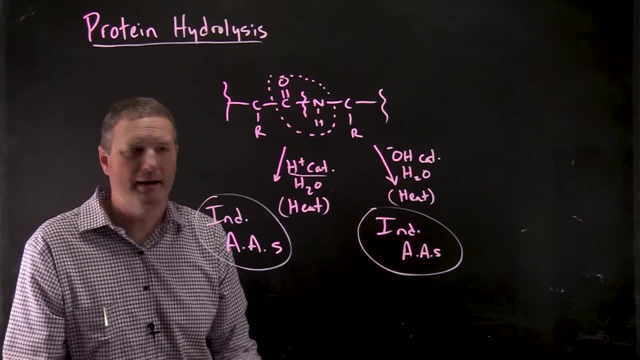 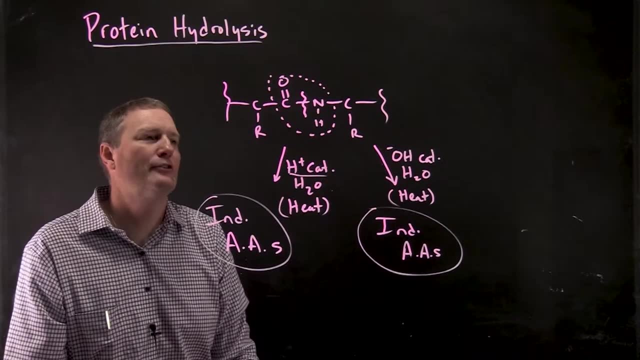 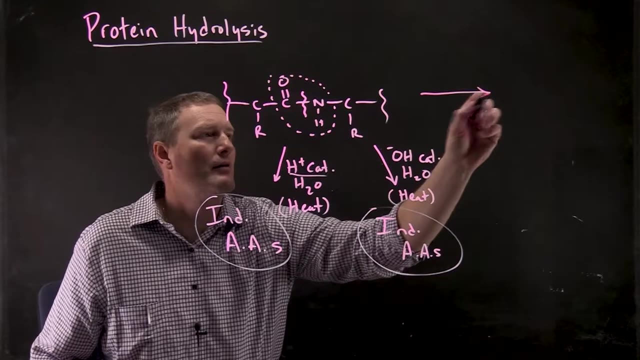 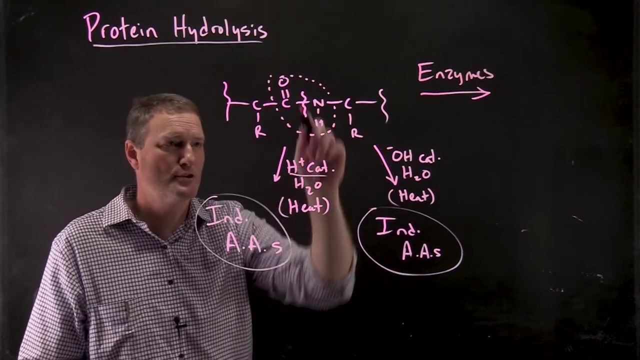 However, in our bodies and in many other circumstances, you don't necessarily need or want to have to treat this with such caustic reagents, And so oftentimes, what's used to degrade a protein are enzymes. okay, and the specific types of enzymes that you can use to break apart. 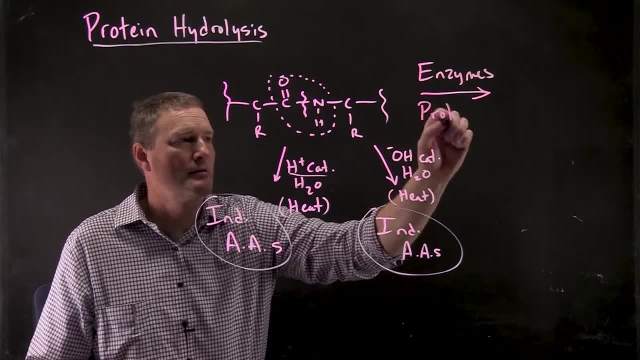 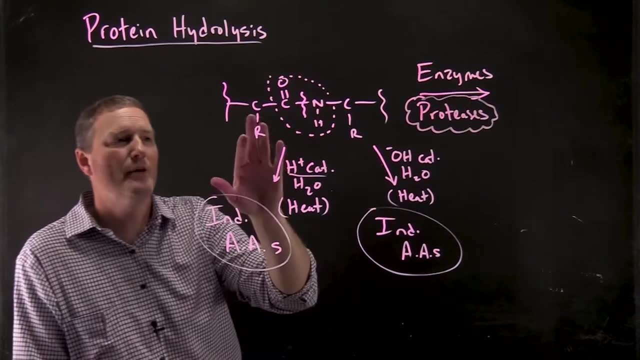 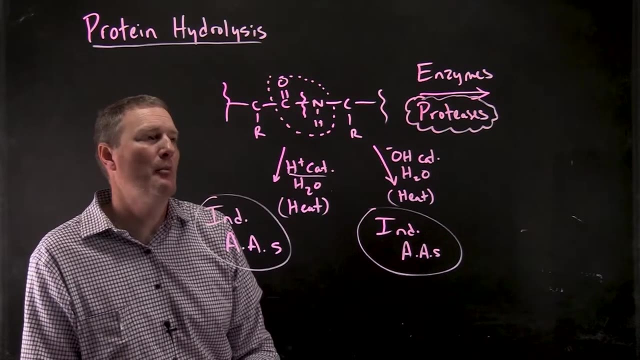 The first one is called the peptide bond. It's a type of bond that's called the protease, And there are a whole host of different proteases that will have different amino acid or sequence specificities. that would allow you to break down specific bonds. 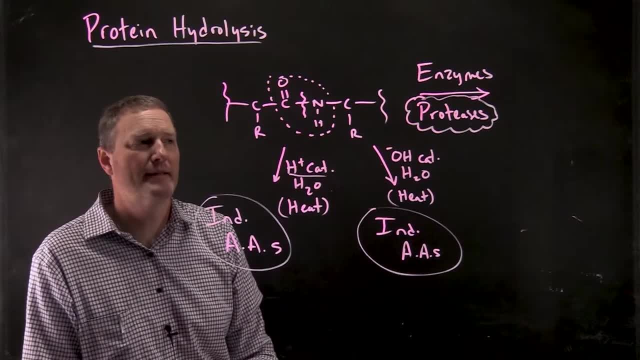 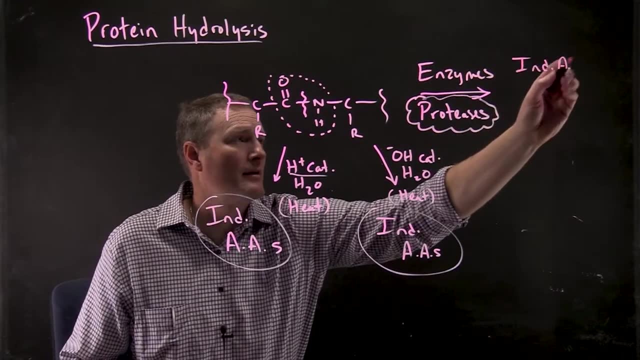 But if you were to treat a peptide like this with a variety of different proteases, you would get individual amino acids and peptide proteins. What's the difference? You would have a broad range of amino acids. You would have a broad range of proteins. 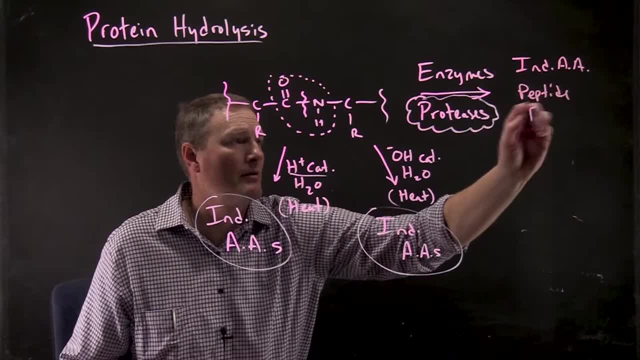 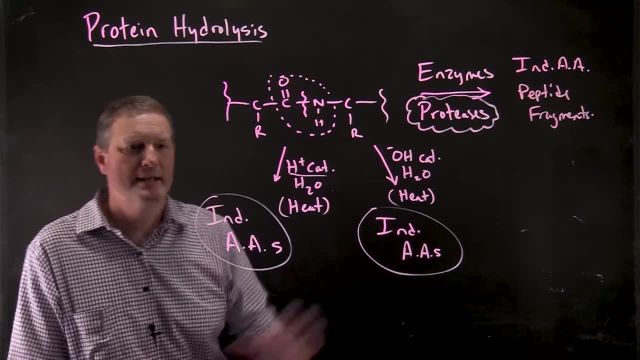 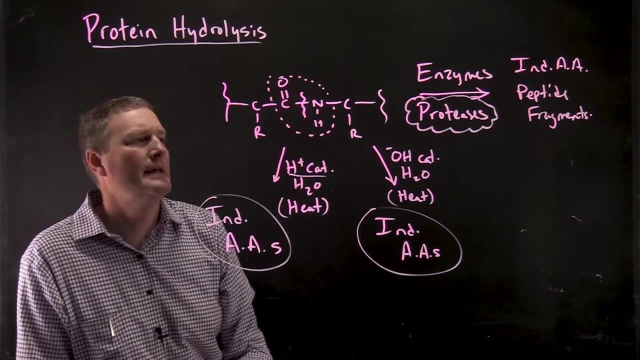 You would have a broad range of amino acids fragments. Okay, because again, if you had a protein of say 300 amino acids, proteases again often have certain specificity. They're only going to cut, say after or before a certain amino acid, So you might not be able to chop the.